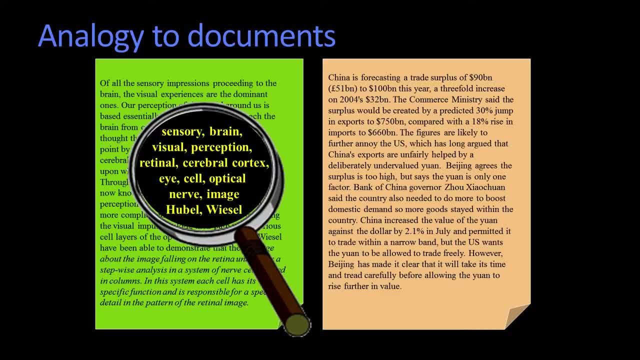 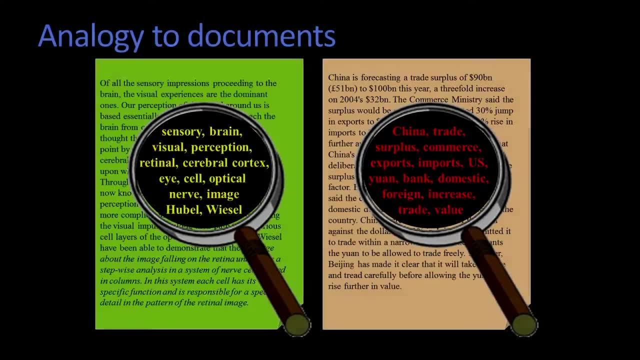 understanding what goes on in the visual cortex of the cat. All right, And here's another document: China trade surplus export Domestic foreign increased trade value. Notice that what's in the magnifying glasses are not ordered. 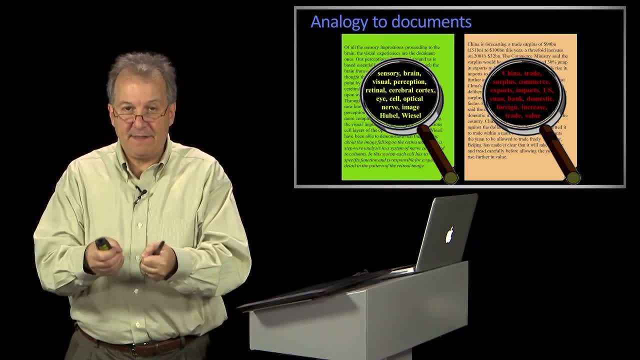 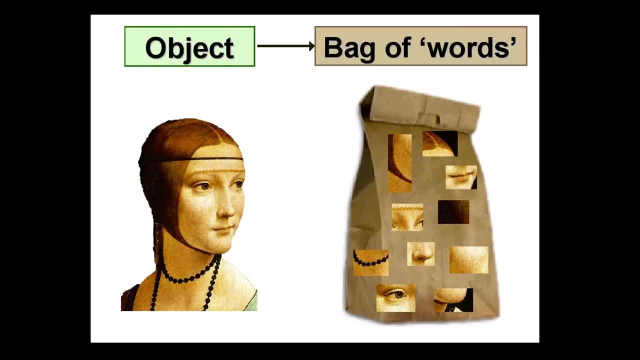 It's just the words that happen to be in that document. It's like you stuck all the words in a bag, And that's where we get this notion of bag of words. okay, And the goal of what we're going to talk about now is to go from object. 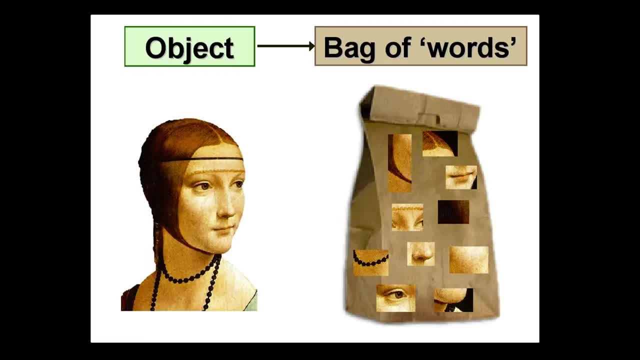 recognition and map that onto a bag of words. And in the document world you know, one way of doing it is I have my bag of words and I say what is the distribution of words in this document? And if I wanted to do document retrieval, I want to find other similar documents. 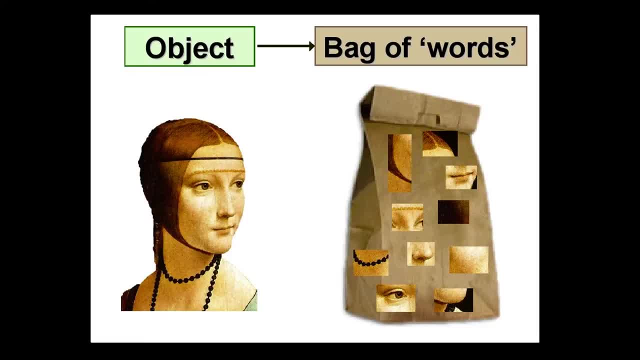 A simple thing you might do is find other documents that have sort of the same histogram distribution of words and that that's likely to be a matching document. Things are much more sophisticated now in terms of how that works, But it's the basic idea is that I've got these code words that represent or 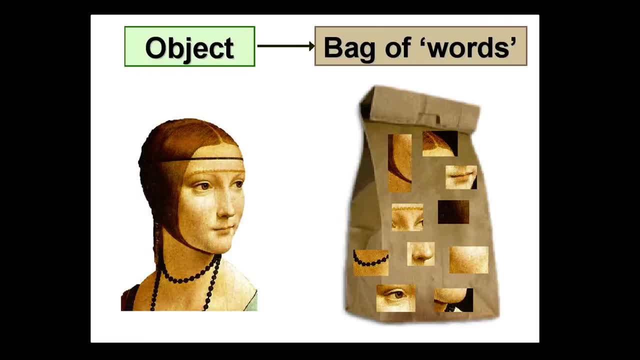 these words that represent something about the semantics, And so a similarity in distribution tells me that maybe there's a good chance that I'm going to have a similar type of document. So we want to do this in computer vision, So that's notionally represented here. 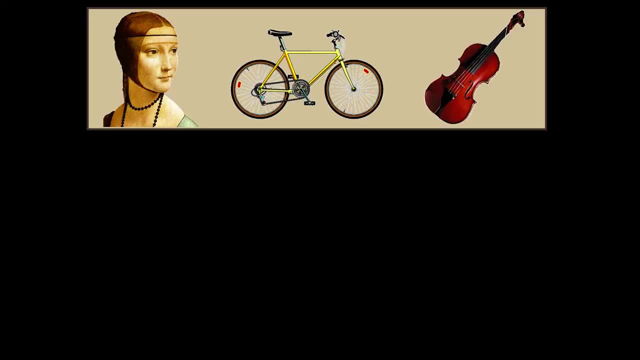 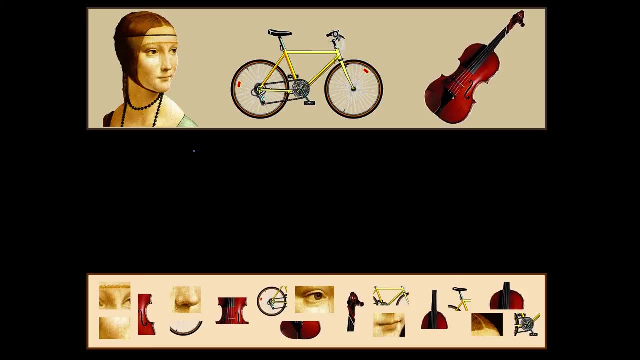 So I've got a bunch of different objects And I compute my features over all of these different objects And I come up with what's shown down here, And I think this slide originally is from Fei-Fei Li. I'm not sure. 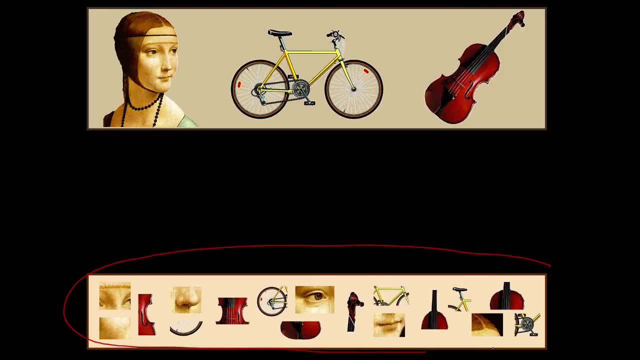 And all of these. these are all of my code words for all of my different objects, right? So I take all my objects and it's kind of like if you take all the documents in a, a library In the United States, and if they're all in English, you took all of those. 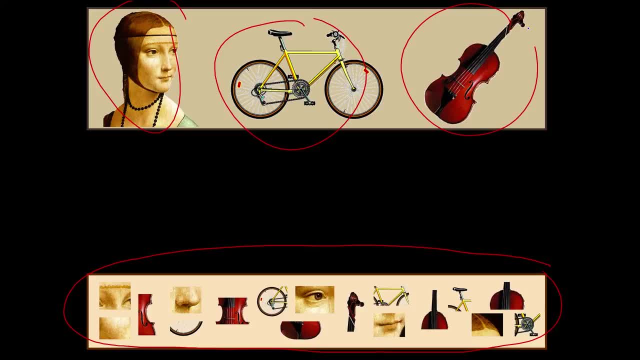 documents together, all of the words would be the set of the words that span all of those documents. right, And in fact there are many more documents than there are words And in fact, if you think of important words, words that actually have a lot of. 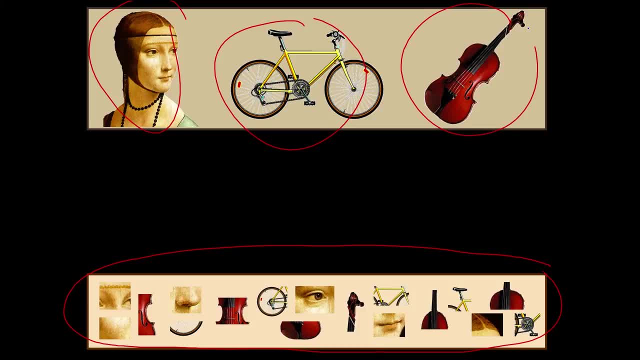 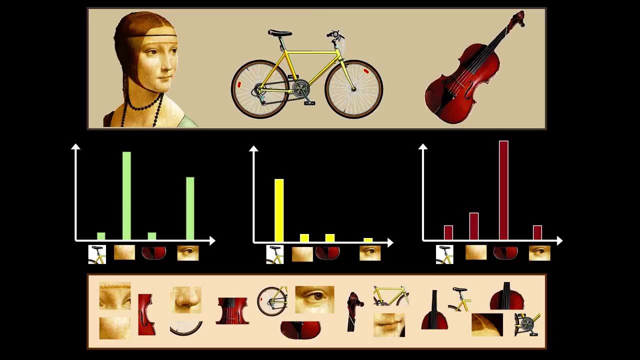 meaning there's way more documents than words. So, given a collection of words, visual words for every document, I can say how many, How many of each word is in each document, And that's what these histograms are meant to represent, right.